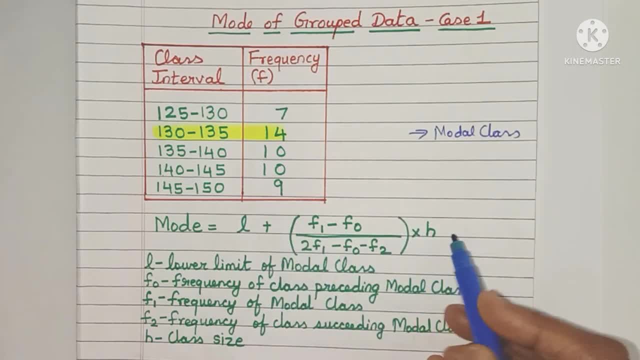 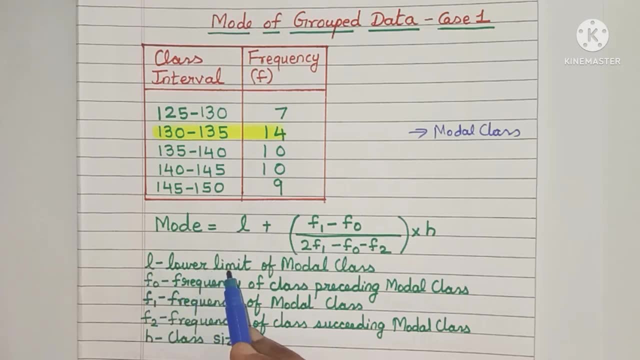 f1 minus f0, minus f2, whole times h. Now, friends, we can easily find all these values now that we know what is the modal class. So L is the lower limit of the modal class. So here is the modal class, friends: 130 to 135.. So the lower limit is 130.. That means my L value will be 130.. Now f0 is: 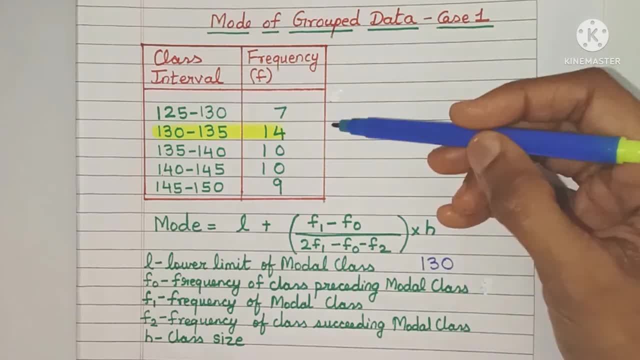 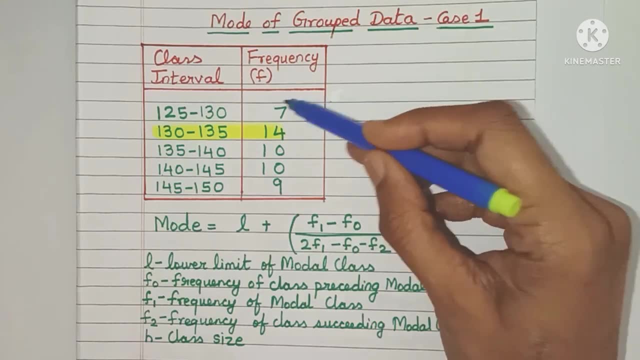 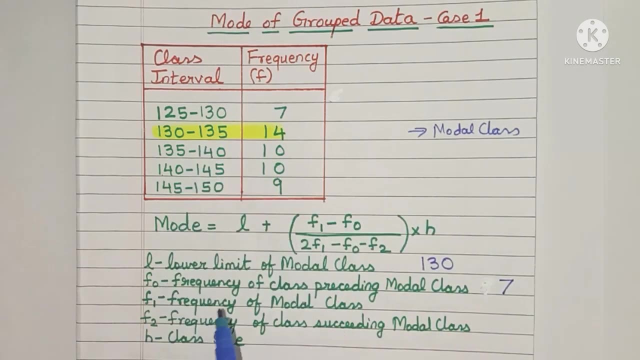 the frequency of the class preceding the modal class. So preceding means coming before, So this is the modal class. So which is the class that comes before the modal class? Yes, this is the class and the frequency of this class is 7.. So f0 will be 7.. So, friends, I hope you understood this. f1 is the frequency. 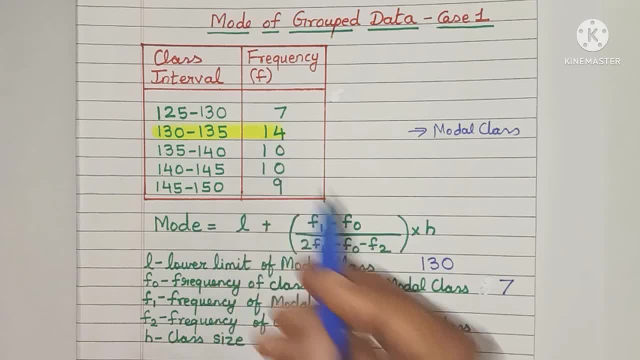 of the modal class. So this is my modal class, whose frequency is 14.. So f1 will be 14. over here Now. f2 is the frequency of the class succeeding the modal class. So succeeding means coming after. So if this is the modal class, the class that comes before the modal class is 14.. So f1 is 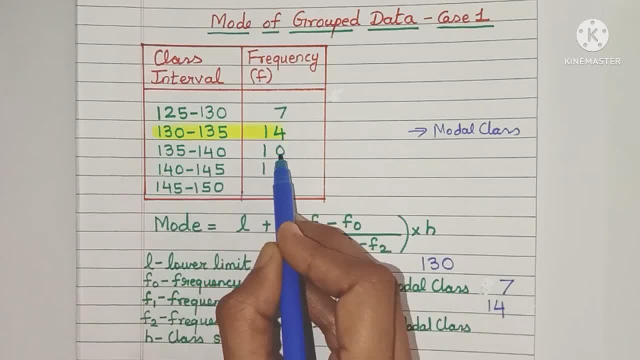 17. Then what comes after the modal class is this class, friends, and the frequency of this class is 10.. That means f2 will be 10.. Now h is the class size, which is very easy to find. Just take any class interval: upper limit minus the lower limit, say here 150 minus 145, and that will give you the 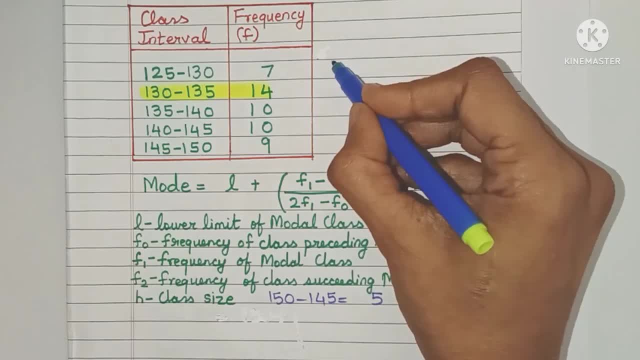 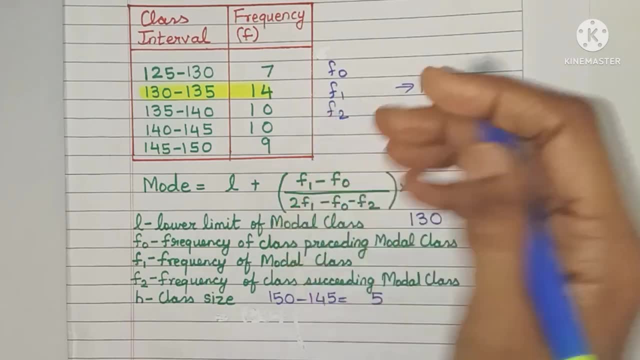 class size, which is 5.. So, friends, just take care while finding the values of the frequencies: f0 will be the frequency of the preceding class, f1 will be the frequency of the modal class, and so on, and F2 will be the frequency of the succeeding class. So don't get confused, friends. Now let's. 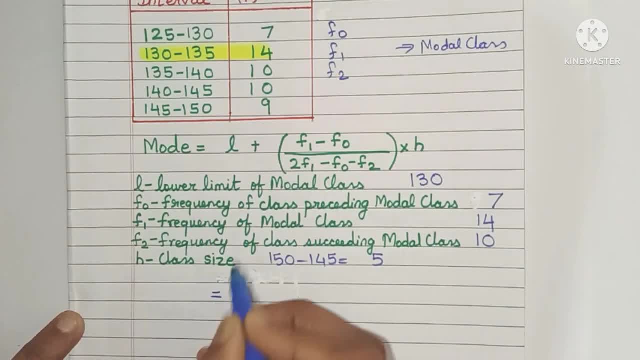 put in all the values in this equation and we will get L as 130 plus F1. minus F0 will be 14 minus 7.. Let's put the bracket 2 times. F1 will be 2 into 14. minus F0 is 7. minus F2 is 10 all. 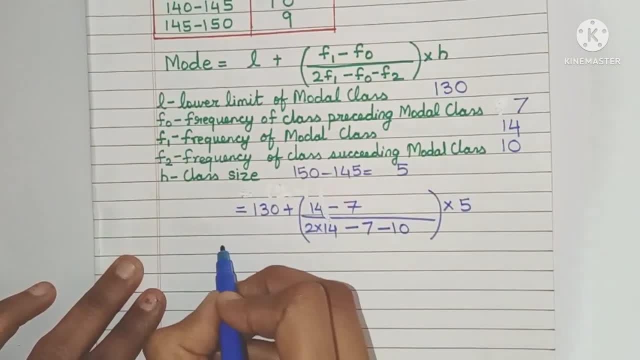 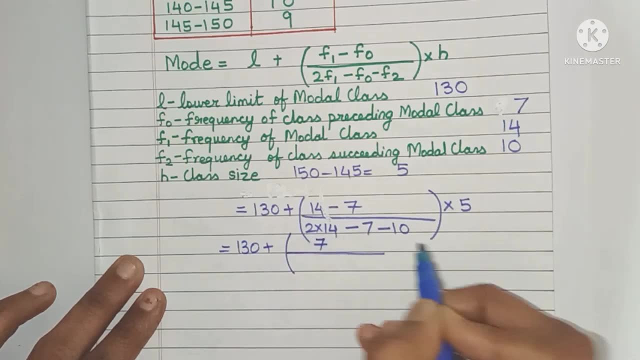 multiplied by H, which is 5.. So let's quickly solve this, friends. We'll get 130 plus. keep the brackets as it is: 7.. 28 minus 7 will be 21.. 21 minus 10 will be 11 times 5.. So, friends, this will be nothing. 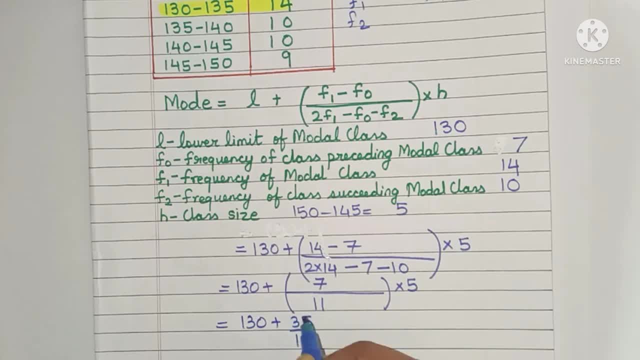 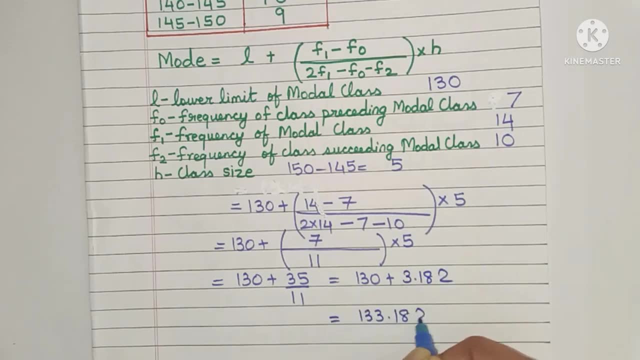 but 130 plus 35 by 11 and 35 by 11 will be nothing but 3.182.. So 133.182, and that is the value of mode. friends, I hope you all have a great day and I will see you in the next video. 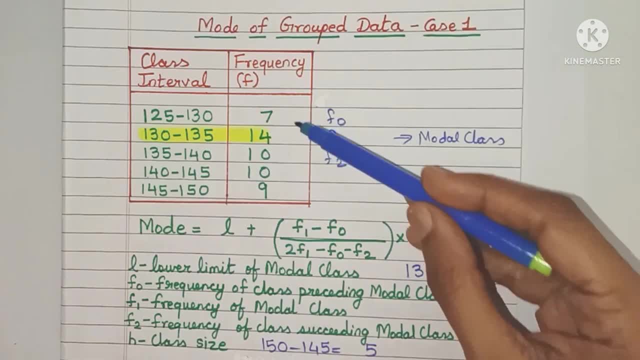 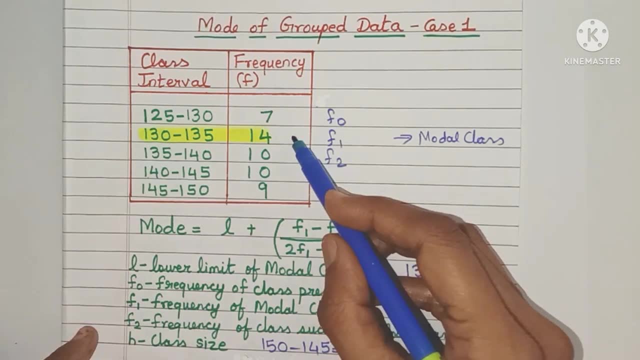 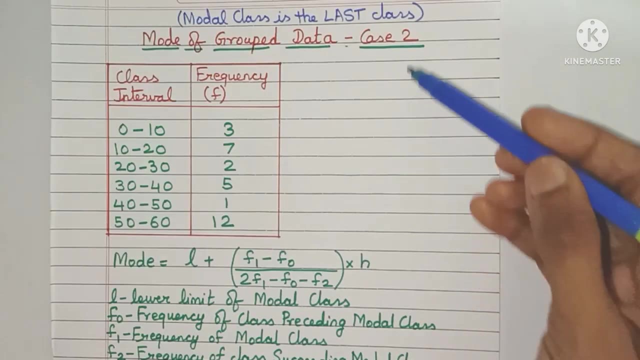 Understood this, friends. Now, friends, in this case the modal class was in between two class intervals, and this is case 1.. But we can have a case where the modal class is the first or the last class. So let's quickly go through those cases also. So let's now consider: 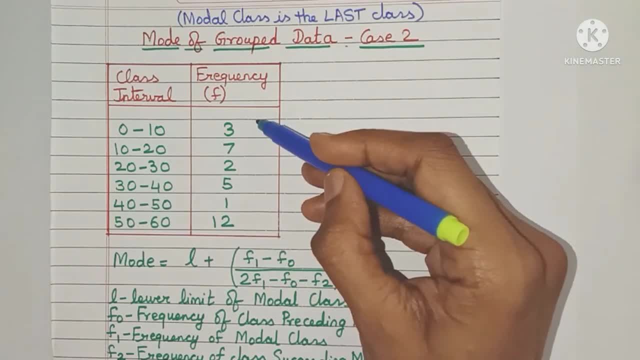 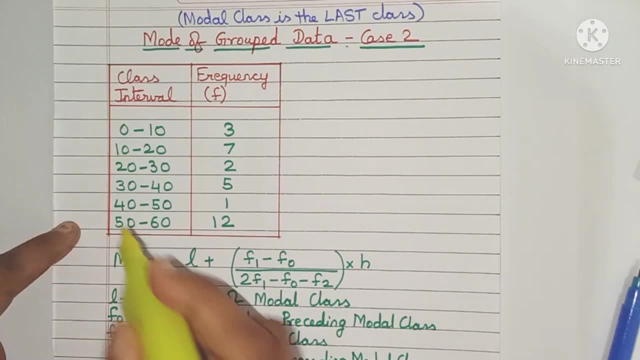 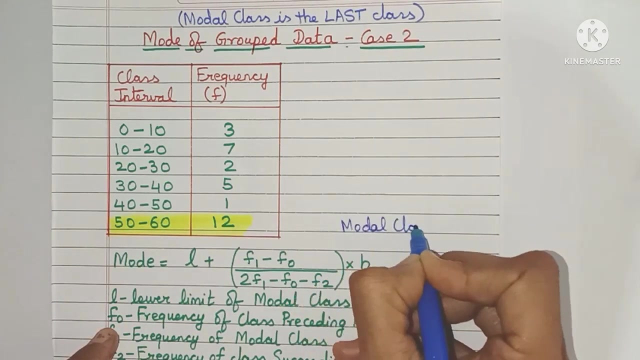 the case where the modal class is the last class. So, as you can see here, 12 is the maximum frequency value, So that means my mode value will also lie here, So let's just highlight it And this will be our modal class, So let's write it over here. So now let's find out the different. 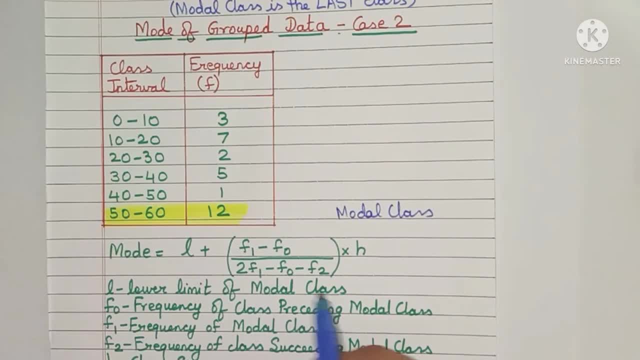 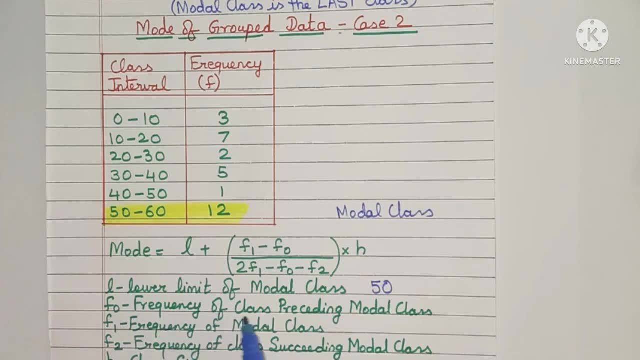 values, friends. L is the lower limit of the modal class, So this is my modal class, and 50 will be the lower limit, So L will be 50.. F0 is the frequency of the class preceding the modal class. So this is my modal class, So the class preceding it will be this class, friends, and its. 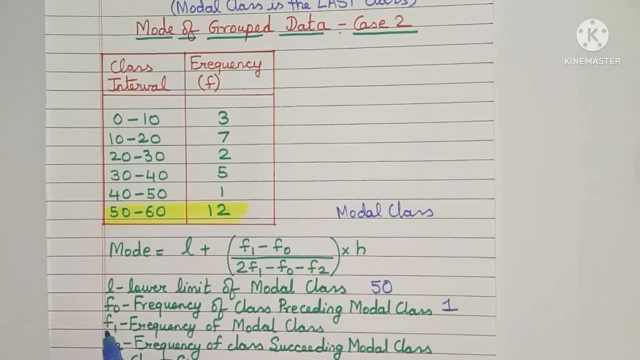 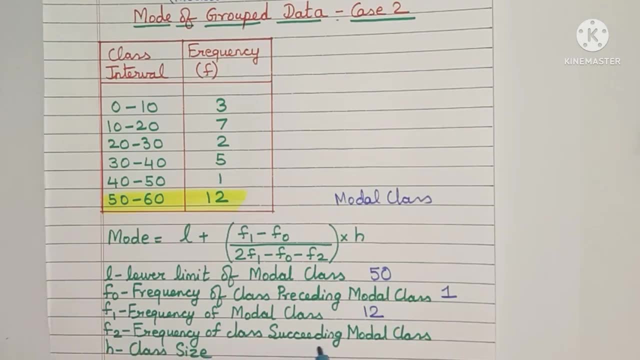 frequency is 1.. So F0 will be 1.. Now, F1 is the frequency of the modal class, So this is my modal class itself, which is 12.. So I'll write it over here. And F2 is the frequency of the class. 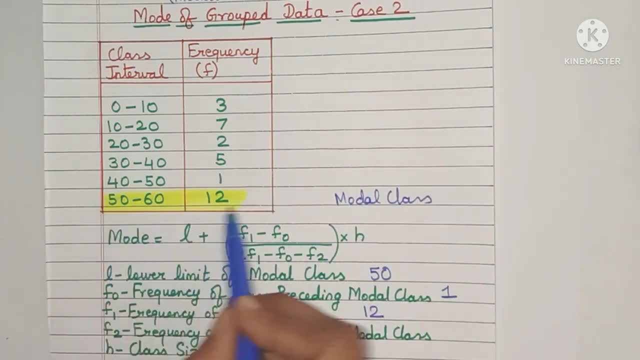 succeeding the modal class. Now, as you can see, friends, this is the modal class, but there is no other class after this modal class. So what should we take as the value of F2?? So in such a case, friends, you should take F2 as 0, because there is no class after it, which means the frequency. 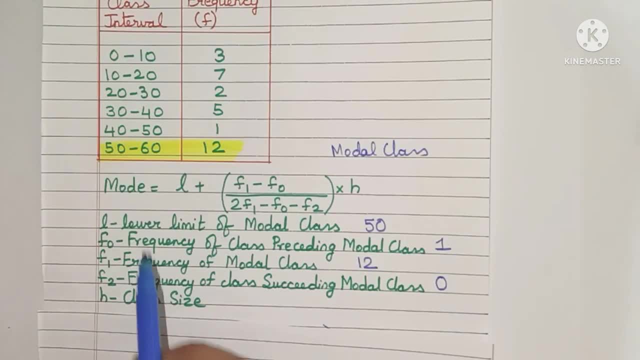 of that class has to be 0.. Now coming to the class size. So just take F2 as 0, because there is no class after it, which means the frequency of that class has to be 0. So let me take any class interval. Let me take 50 minus 40. I will get the answer as 10.. So H is 10. 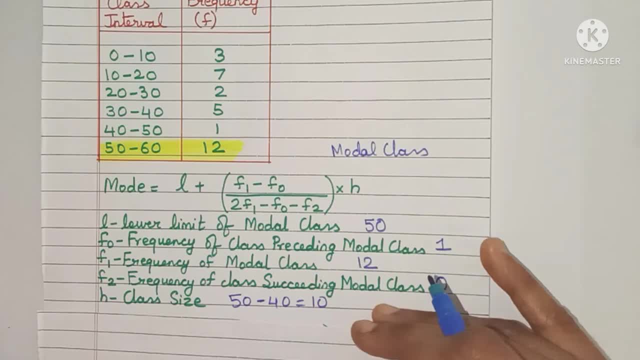 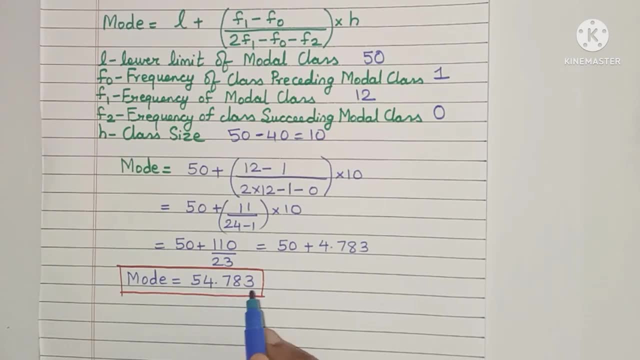 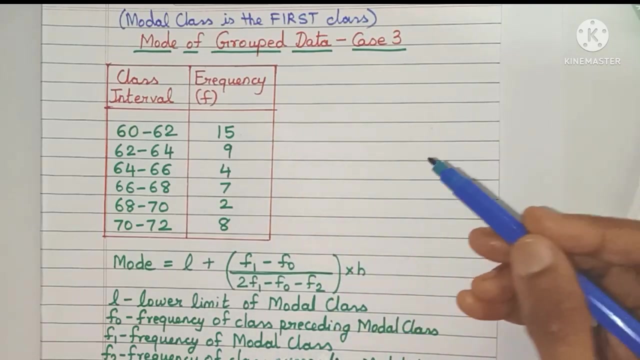 friends, Now you just need to follow the same procedure, putting in all the values in this formula. So, friends, I have already done that and I got the mode value as 54.783.. Now let's come to the last case, friends. Here again, let's first find the frequency, which is maximum, As you can see.